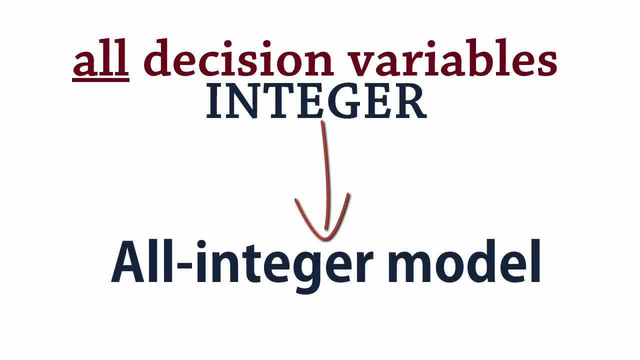 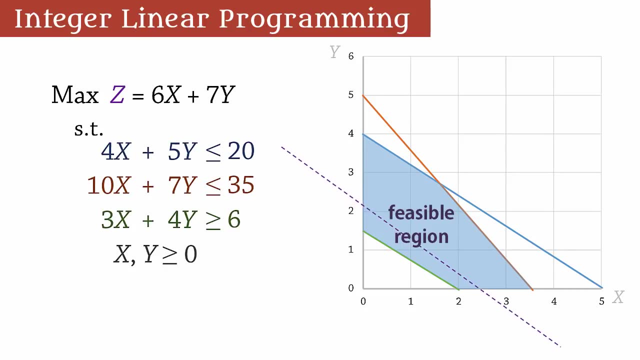 required to be integer. we refer to that as an all integer model, also referred to as pure or total integer model. Consider this LP model and its graph. Here is the feasible region Moving the objective function line upwards. since this is a maximization problem, we see that the optimal solution occurs here. 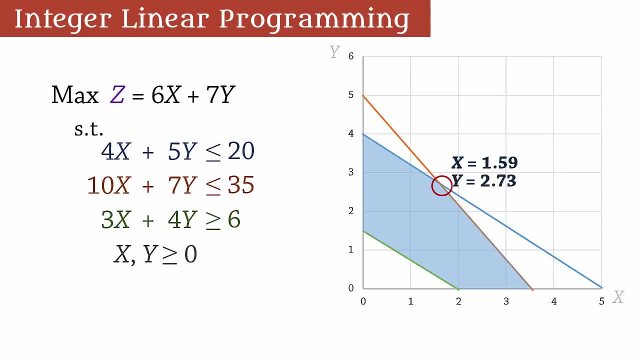 at X equals 1.59 and Y equals 2.73.. With a constant of 1.59, we see that the optimal solution occurs here: at X equals 1.59 and Y equals 2.73, with a corresponding objective function value of 28.65.. Now suppose x actually represents the number of 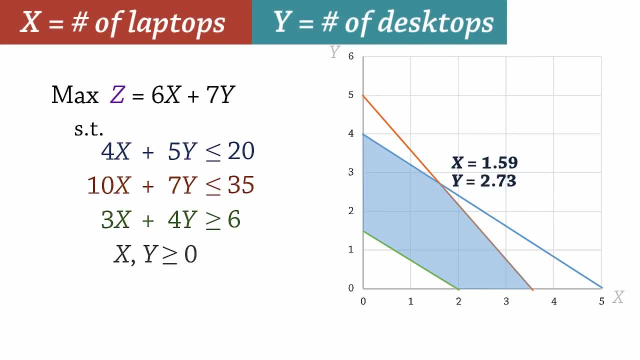 laptops and y the number of desktops to purchase for a new office. Since, by definition, x and y can only assume integral values or whole numbers, this is an all-integer model. So to indicate that we append the term an integer to the model, The feasible solutions are now reduced only to the 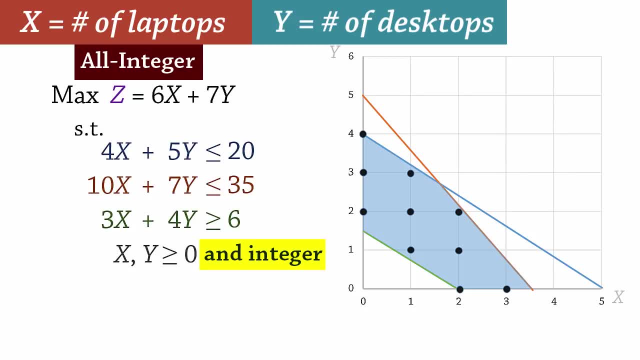 point where both x and y are integers simultaneously. It follows that the feasible solutions to an all-integer problem are a collection of dots. Moving the objective function line upwards, we see that the optimal solution to the all-integer problem occurs here, at 0,4,. 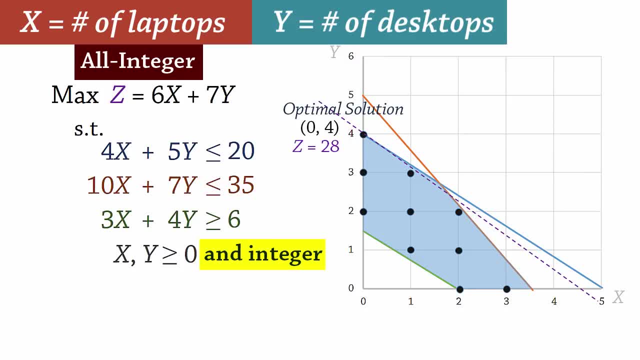 with an objective function value of 28.65.. So the optimal solution to the all-integer problem occurs here at 0,4, with an objective function value of 28.65.. That is, purchase no laptops and four desktops for. 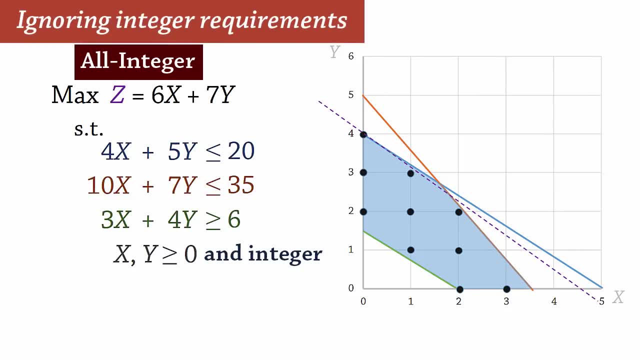 the office. Now suppose we decide to ignore or relax the integer requirement and use the best optimal solution satisfying the constraints which we saw earlier on. We refer to that as LP relaxation. So LP relaxation simply means that we begin with an integer problem and later. 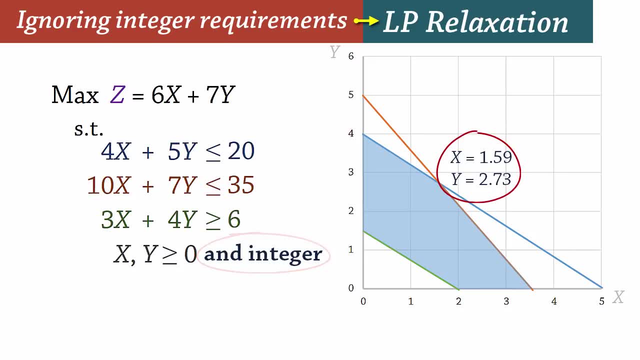 ignore the integer requirements when finding the solution. As a result, LP relaxation always provides an upper bound for the optimal value in a maximization integer problem. In other words, the optimal value produced by an integer problem cannot be better than that of its corresponding LP relaxation problem, That is, for a maximization. 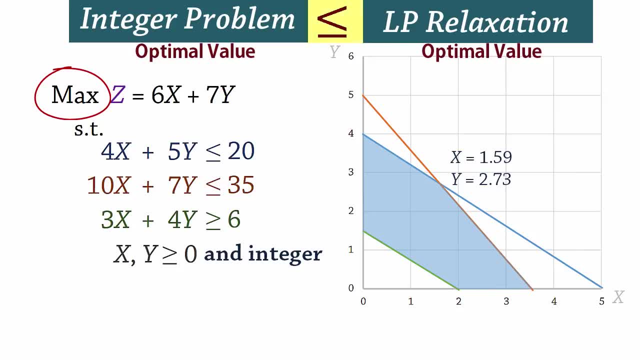 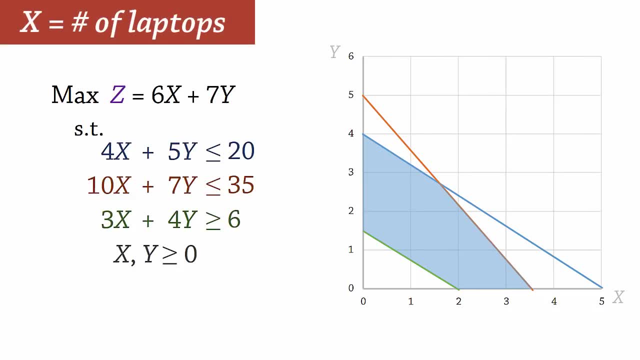 problem. the optimal value of the integer problem will be less or equal to that of its LP relaxation. X is still the number of laptops to purchase, but Y is now the amount of time spent on the laptops. Because only X now needs to be integer, we append an X integer to the model Since 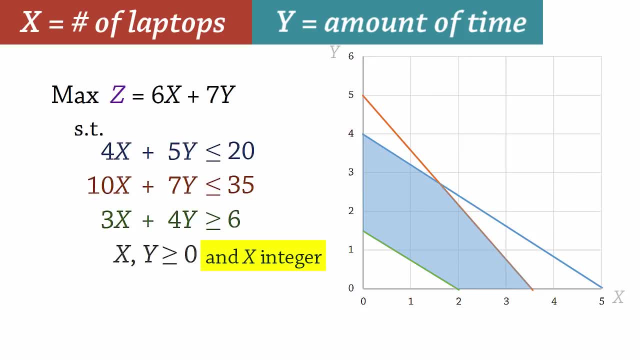 not all decision variables need to be integer. we refer to this as a mixed integer problem. The feasible solutions are now a set of vertical lines showing that X must be an integer and Y can assume any value. So if we move the objective function line upwards, we see that the optimal solution 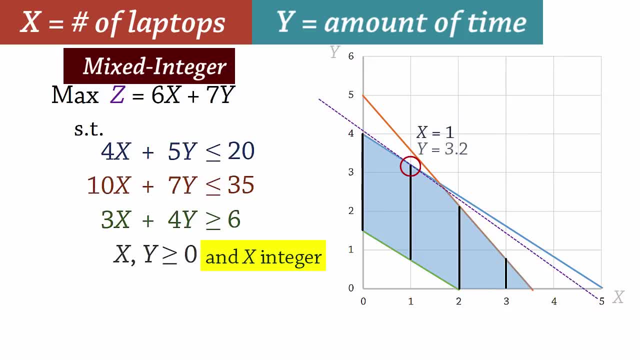 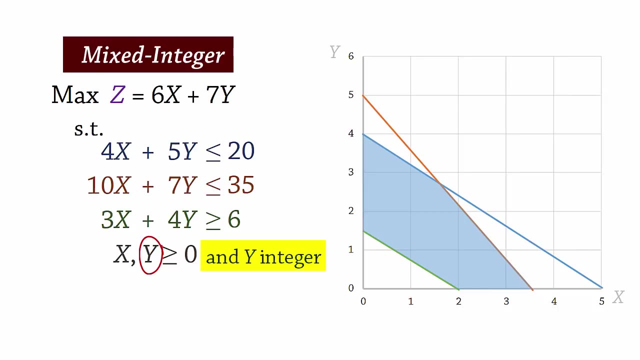 occurs here at X equals 1 and Y equals 3.2, with a corresponding optimal value of Z equals 28.4.. Suppose instead only Y is required to be an integer and not X. Then we have another mixed integer problem. In this case, the feasible solutions would be a set of horizontal lines. 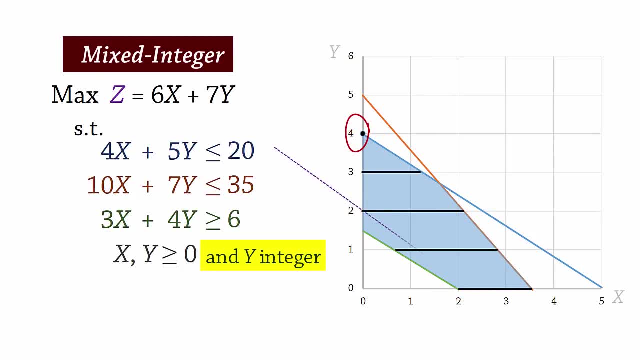 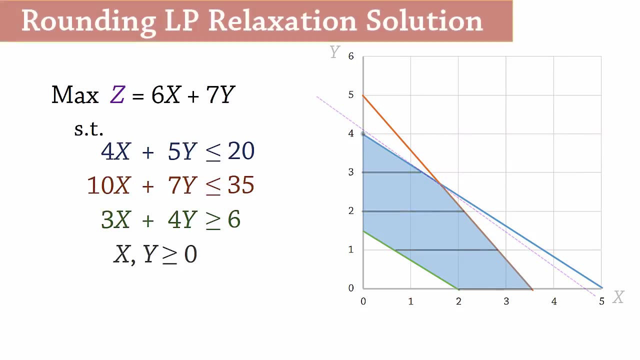 including this point here at 0.4.. Moving the objective function line again, we see that the optimal solution occurs here at X equals 1.25 and Y equals 3, with an objective function value of 28.5.. Let's now examine what could happen when we round the optimal solution to the LP relaxation. 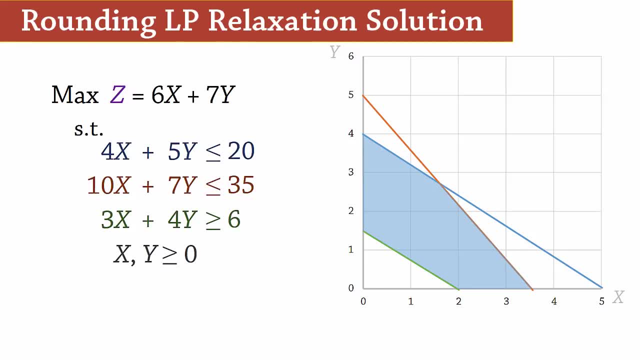 to an integer solution. Recall that the optimal solution to the LP relaxation problem is X equals 1.59 and Y equals 0.5.. The optimal solution to the LP relaxation problem is Y equals 2.73, with an optimal objective function value of 28.65.. 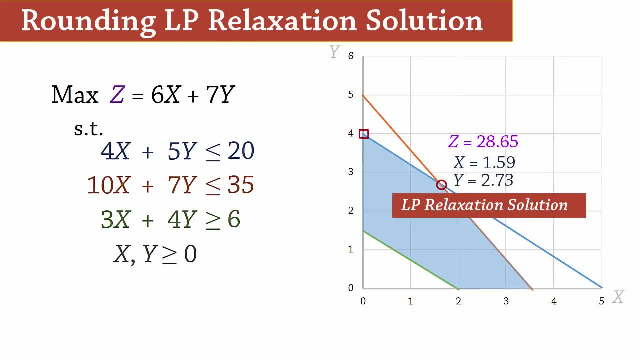 Recall also that the optimal all-integer solution occurs here at 0.4.. Rounding down the LP: relaxation solution gives X equals 1 and Y equals 2, which is a feasible solution but not optimal. So as long as the coefficients in a maximization problem are positive, rounding down the LP.